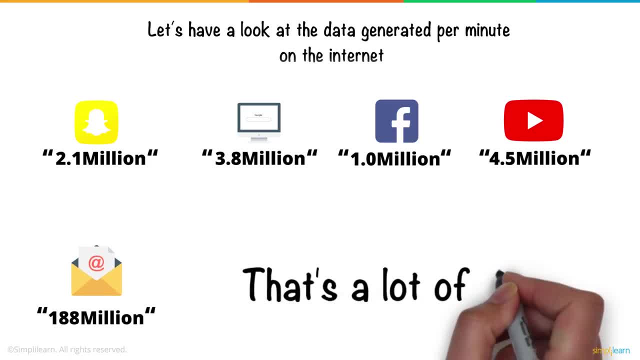 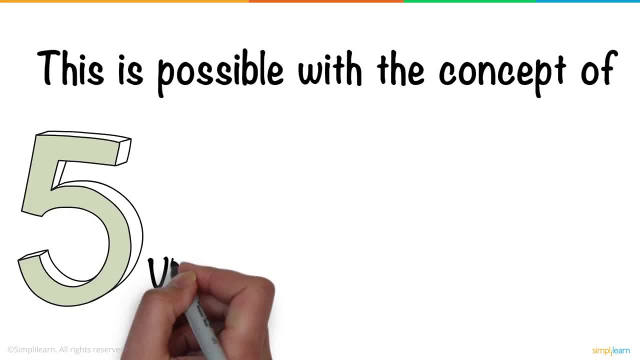 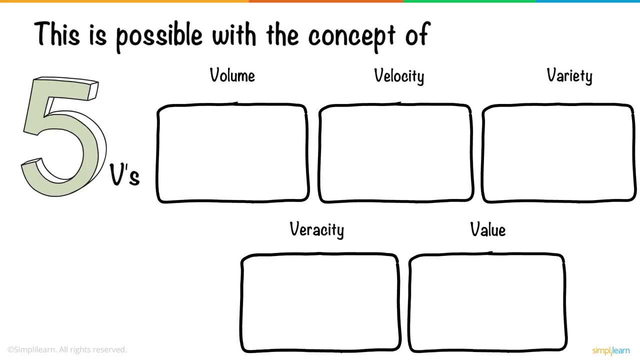 188 million emails are sent. That's a lot. So how do you classify any data as big data? This is possible with the concept of five Vs: Volume, velocity, variety, veracity and value. Let us understand this with an example from the healthcare industry. 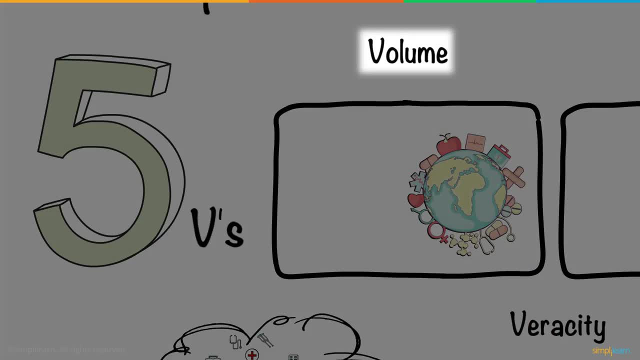 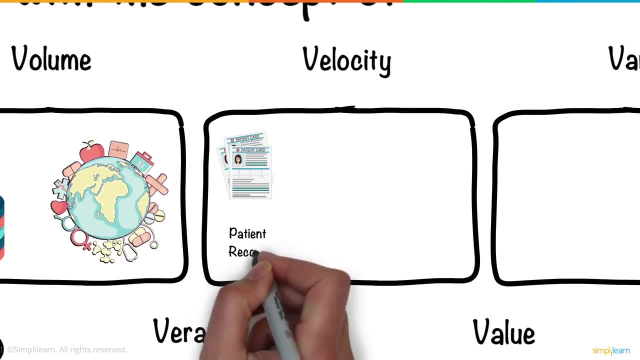 Hospitals and clinics across the world generate massive volumes of data. 2,314 exabytes of data are collected annually in the form of patient records and test results. All this data is generated at a very high speed, which attributes to the velocity of big data. 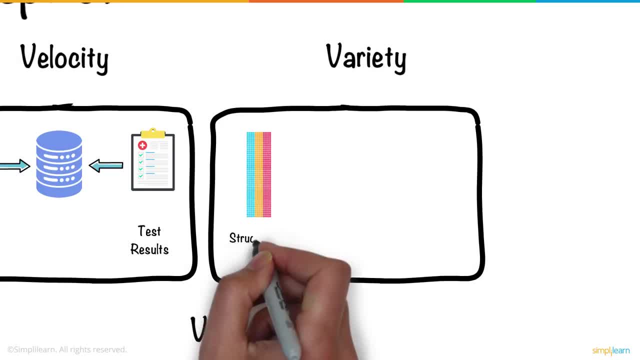 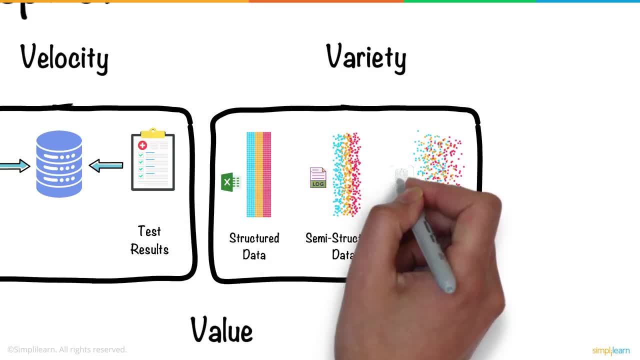 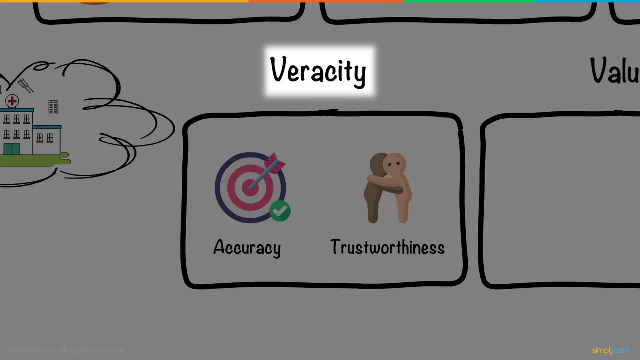 Variety refers to the various data types, such as structured, semi-structured and unstructured data. Examples include Excel records, log files and X-ray images. Accuracy and trustworthiness of the generated data is termed as veracity. Analyzing all this data will benefit the medical sector by enabling faster disease detection. 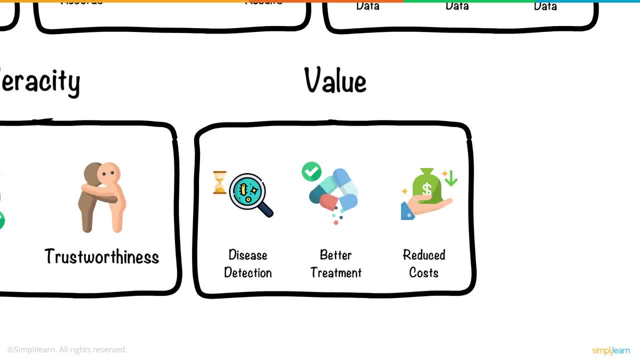 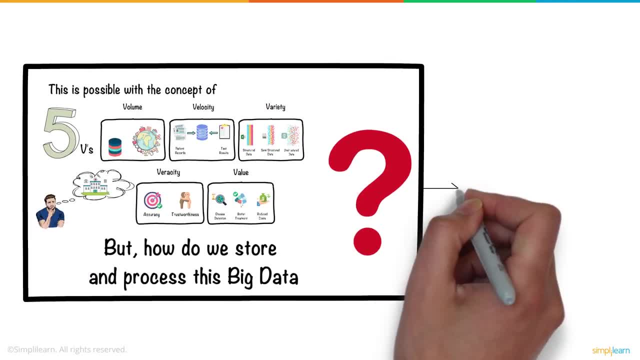 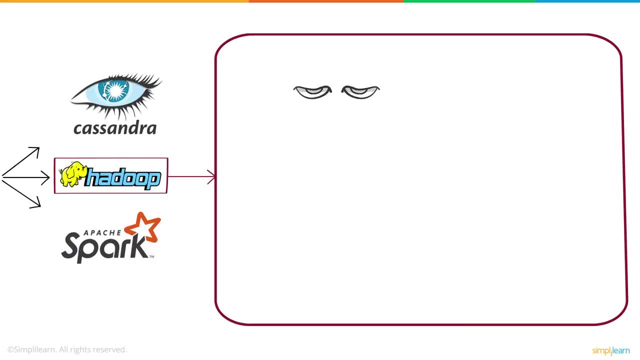 better treatment and reduced cost. This is known as the value of big data. But how do we store and process this big data? To do this job, we have various frameworks, such as Cassandra, Hadoop and Spark. Let us take Hadoop as an example and see how Hadoop stores and processes big data. 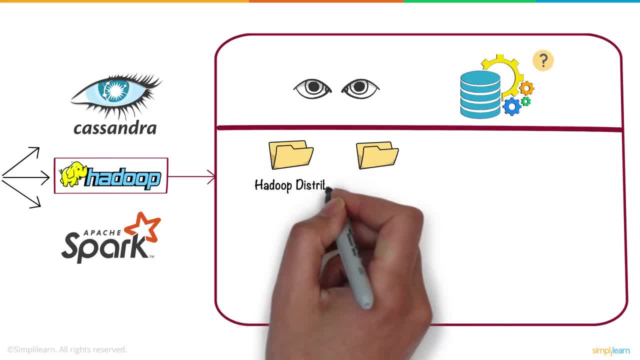 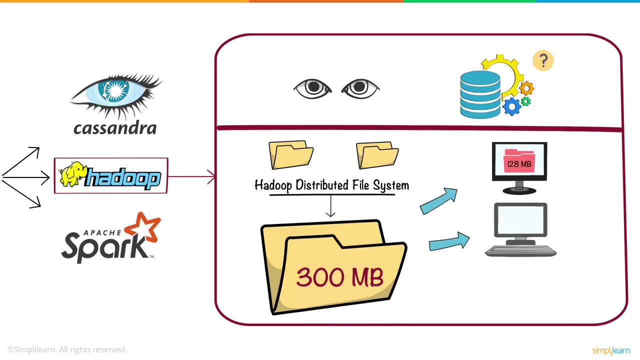 Hadoop uses a distributed file system, known as Hadoop Distributed File System, to store big data. What is Hadoop? If you have a huge file, your file will be broken down into smaller chunks and stored in various machines. Not only that, when you break the file, you also make copies of it, which goes into different nodes. 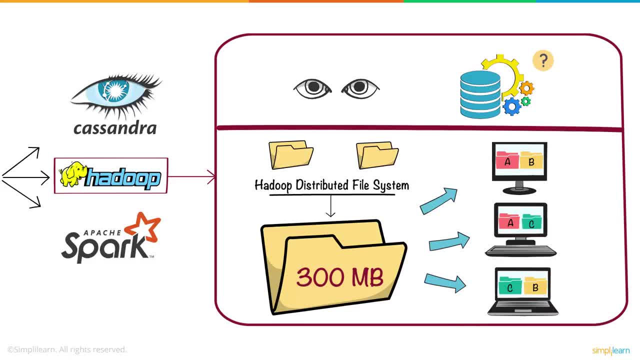 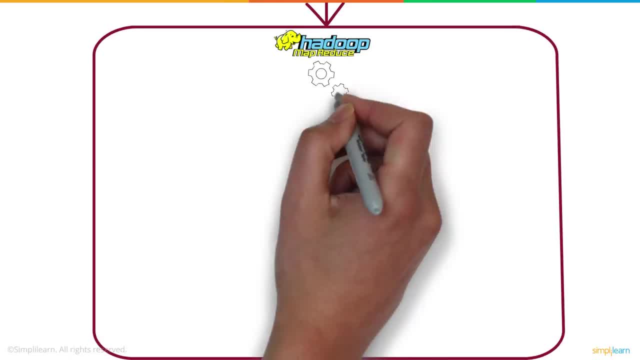 This way, you store your big data in a distributed way And make sure that even if one machine fails, your data is safe on another. Map-reduce technique is used to process big data. A lengthy task A is broken into smaller tasks. 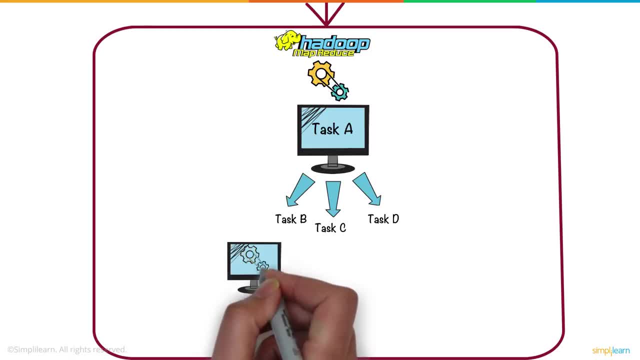 B, C, D, E and Z. Now, instead of one machine, three machines take up each task and complete it in a parallel fashion and assemble the results at the end. Thanks to this, the processing becomes easy and fast. This is known as parallel processing. 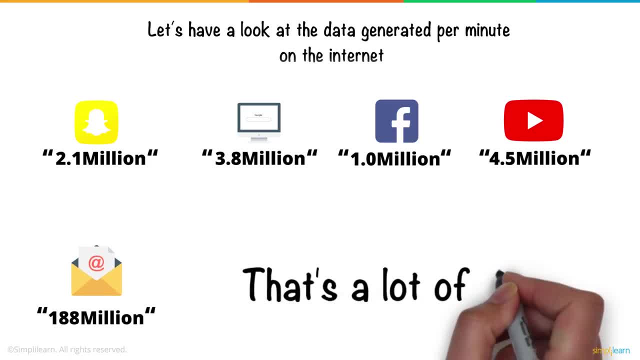 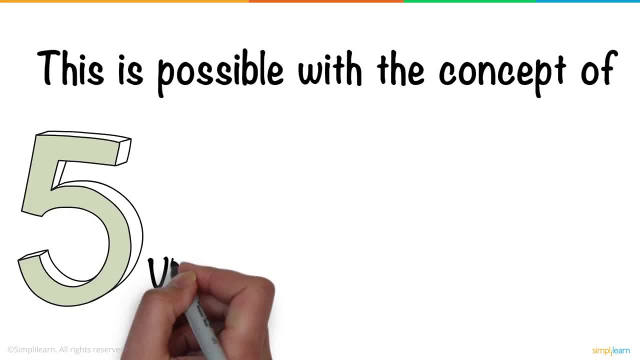 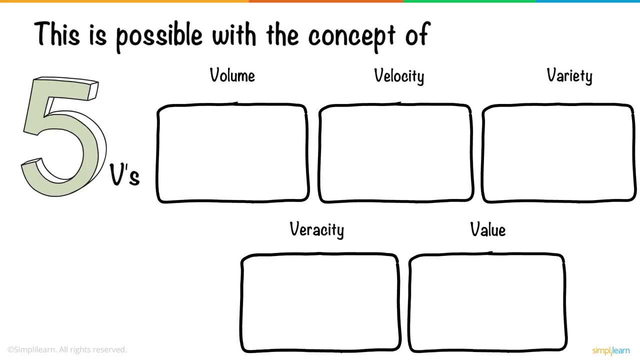 188 million emails are sent. That's a lot. So how do you classify any data as big data? This is possible with the concept of five Vs: Volume, velocity, variety, veracity and value. Let us understand this with an example from the healthcare industry. 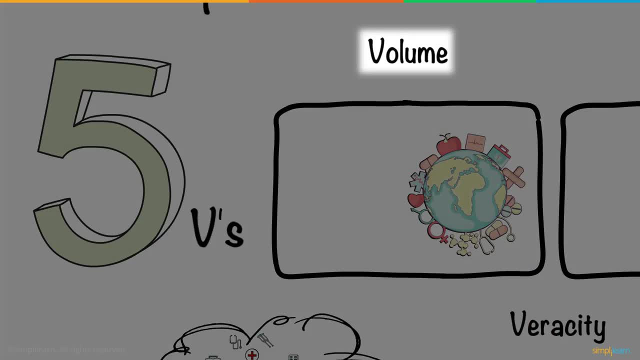 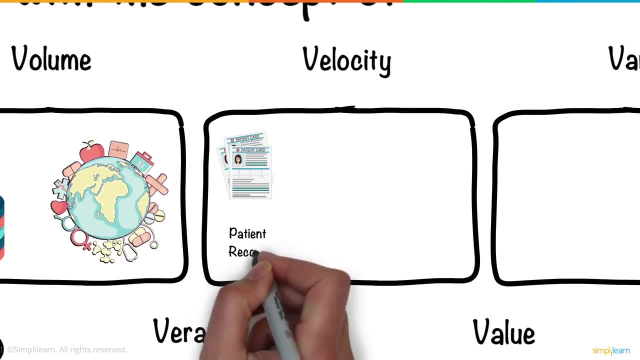 Hospitals and clinics across the world generate massive volumes of data. 2,314 exabytes of data are collected annually in the form of patient records and test results. All this data is generated at a very high speed, which attributes to the velocity of big data. 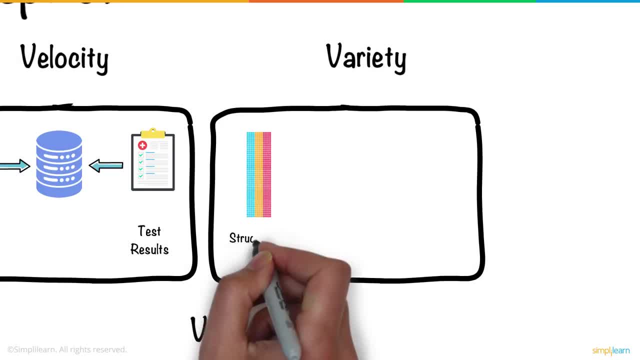 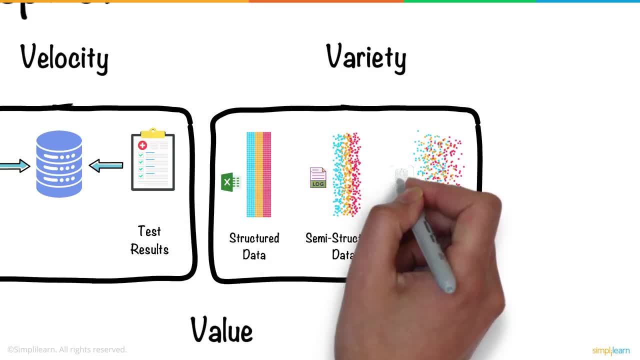 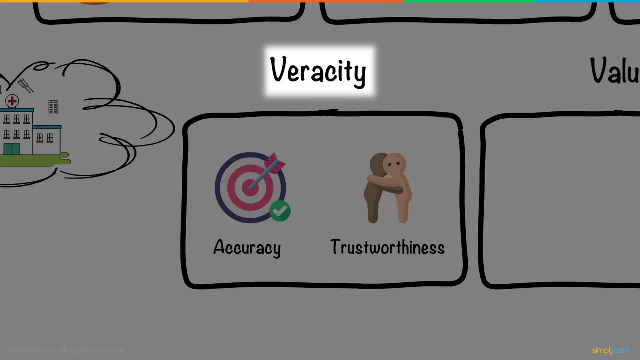 Variety refers to the various data types, such as structured, semi-structured and unstructured data. Examples include Excel records, log files and X-ray images. Accuracy and trustworthiness of the generated data is termed as veracity. Analyzing all this data will benefit the medical sector by enabling faster disease detection. 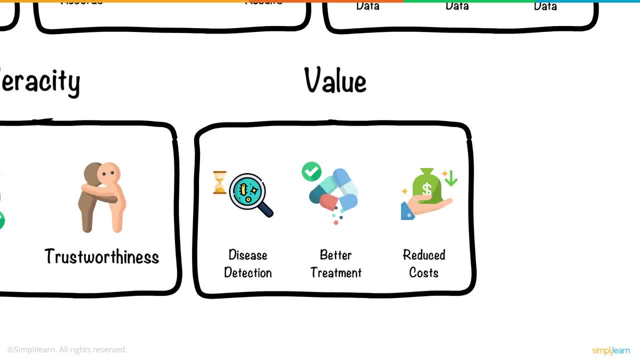 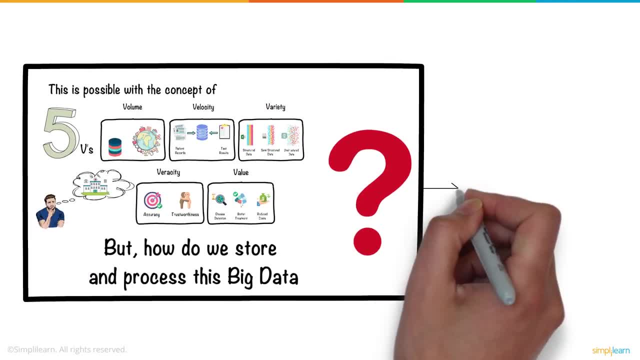 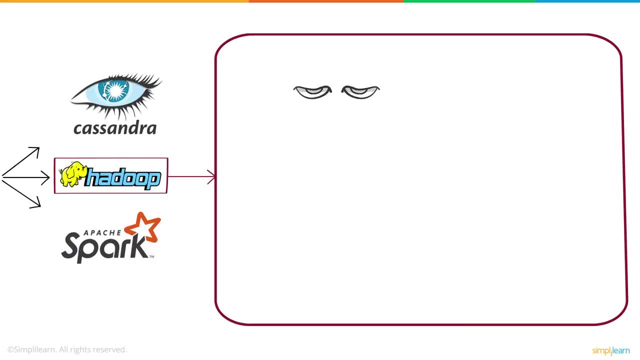 better treatment and reduced cost. This is known as the value of big data. But how do we store and process this big data? To do this job, we have various frameworks, such as Cassandra, Hadoop and Spark. Let us take Hadoop as an example and see how Hadoop stores and processes big data. 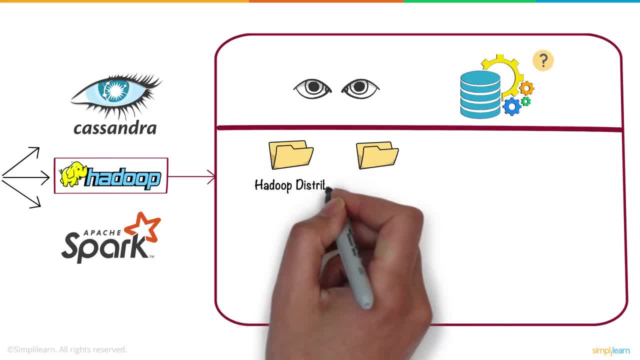 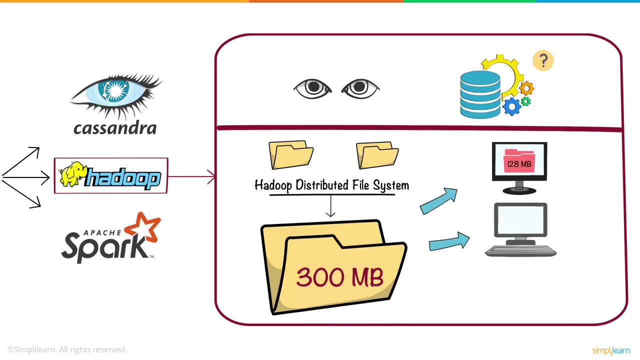 Hadoop uses a distributed file system, known as Hadoop Distributed File System, to store big data. What is Hadoop? If you have a huge file, your file will be broken down into smaller chunks and stored in various machines. Not only that, when you break the file, you also make copies of it, which goes into different nodes. 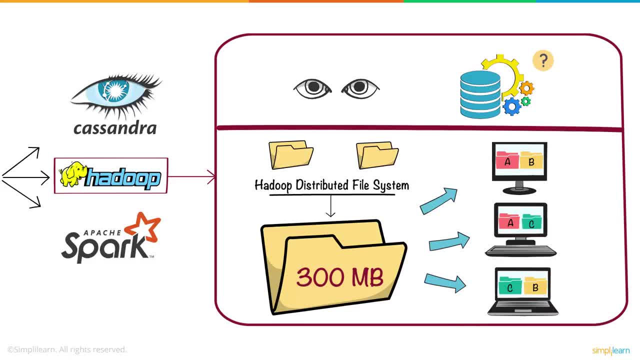 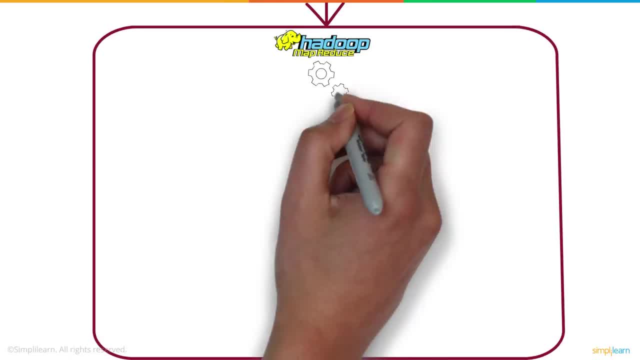 This way, you store your big data in a distributed way And make sure that even if one machine fails, your data is safe on another. Map-reduce technique is used to process big data. A lengthy task A is broken into smaller tasks. 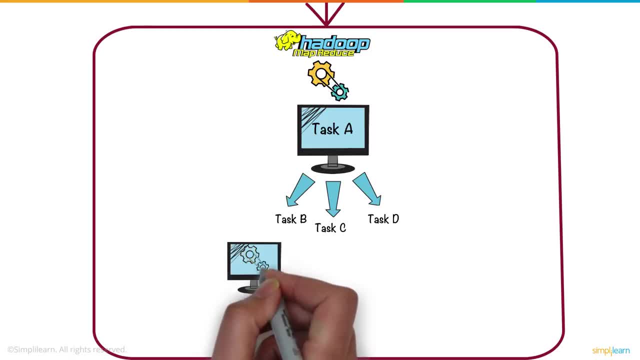 B, C, D, E and Z. Now, instead of one machine, three machines take up each task and complete it in a parallel fashion and assemble the results at the end. Thanks to this, the processing becomes easy and fast. This is known as parallel processing.